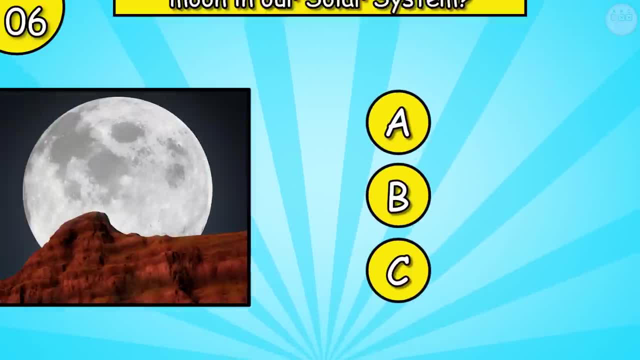 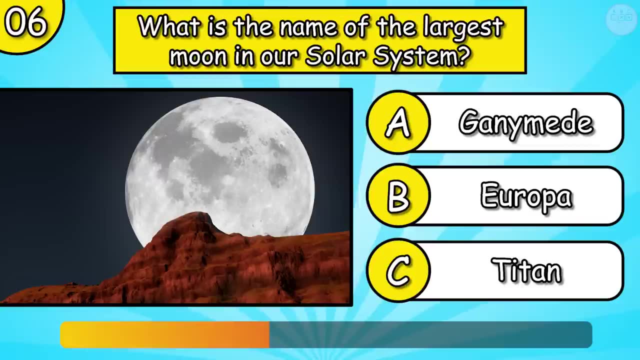 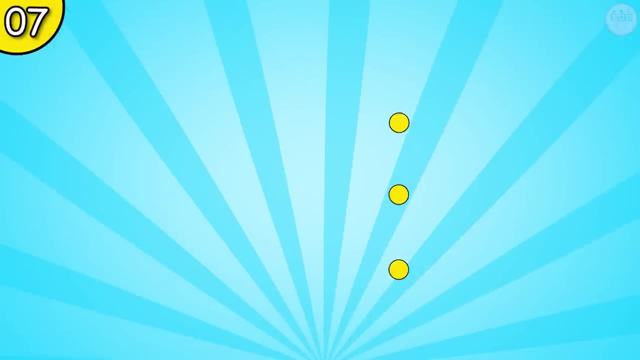 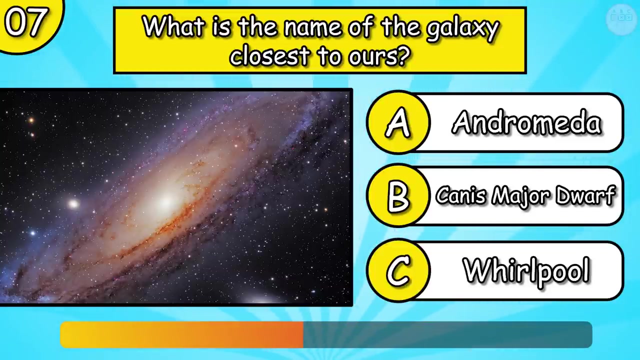 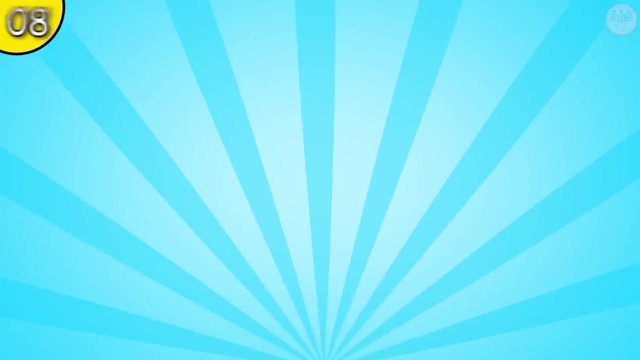 It's Sirius. What is the name of the largest moon in our solar system, Ganymede? What is the name of the galaxy closest to ours? It's Canis Major Dwarf. What's the name of the belt of asteroids between Mars and Jupiter? Mars and Jupiter. 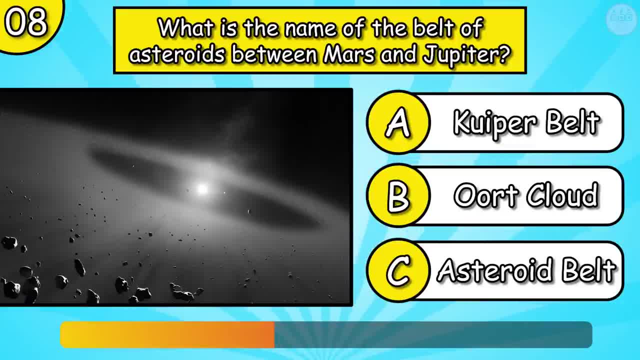 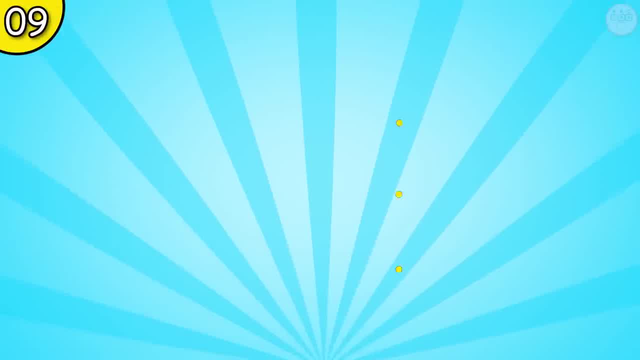 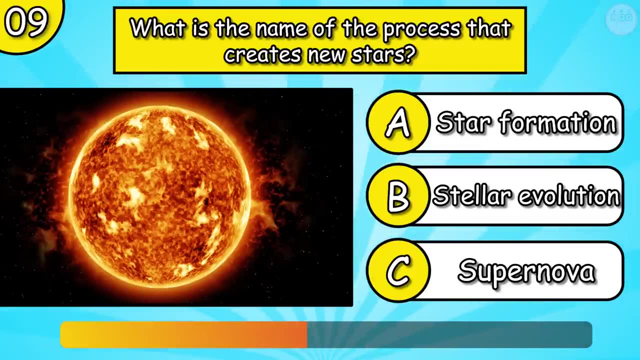 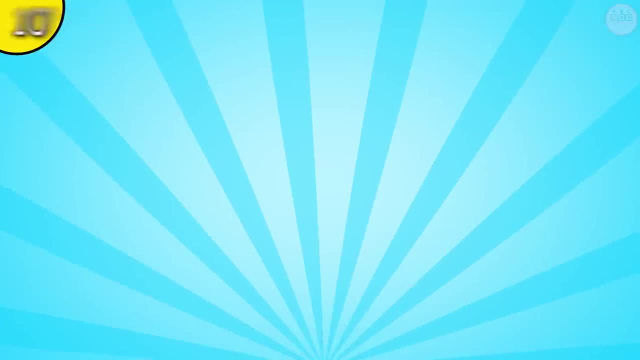 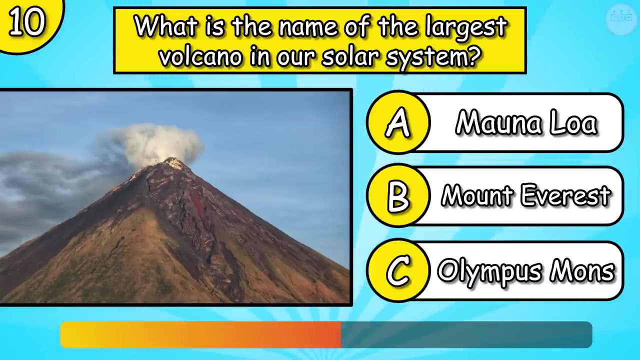 What is the name of the largest planet in the world, Jupiter? What's the name of the last star in the world, Mars and Jupiter? It's asteroid belt. What's the name of the process that creates new stars? It's star formation. What's the name of the largest volcano in our solar system? 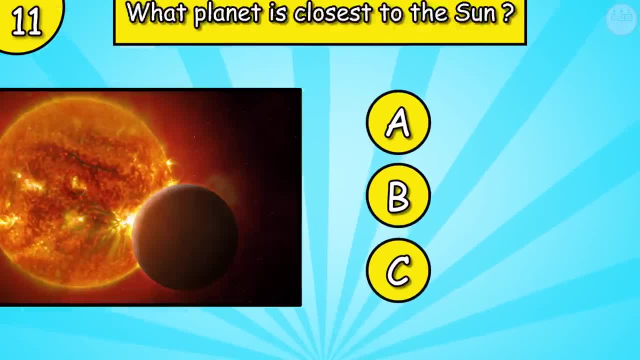 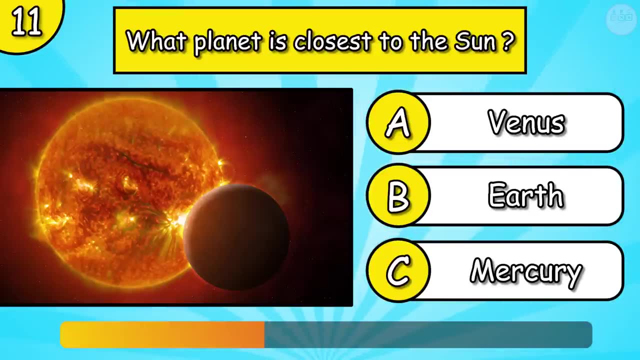 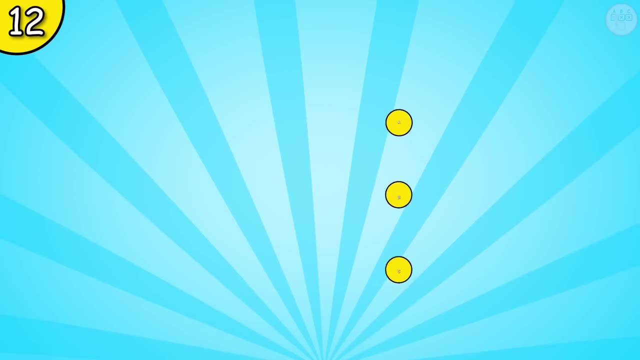 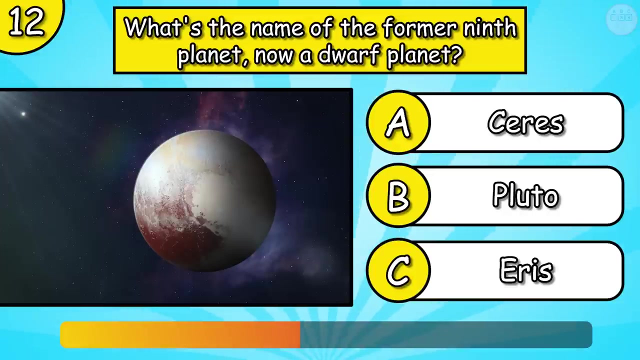 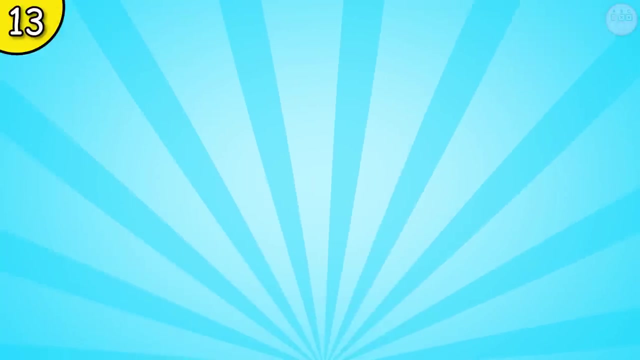 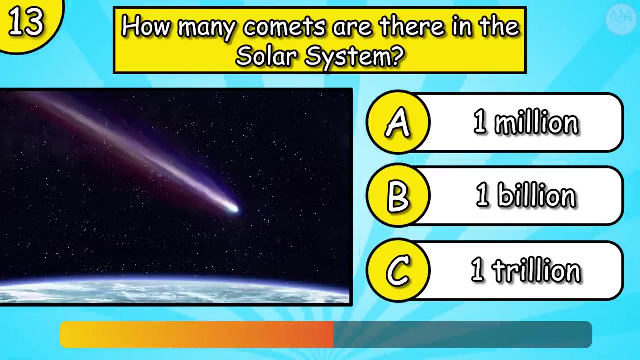 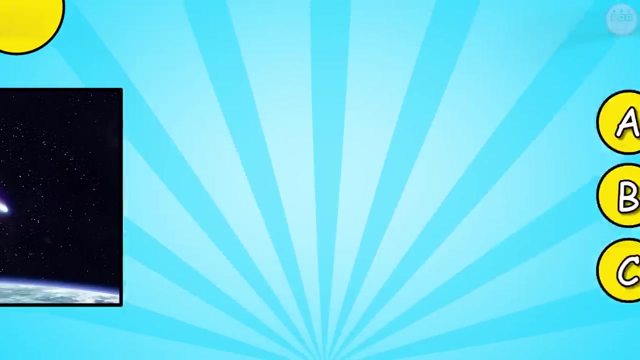 It's Olympus Mons. What planet is closest to the Sun? It's Mercury. What's the name of the former ninth planet, now a dwarf planet? It's Pluto. How many comets are there in the solar system? One trillion. What planet is closest to Saturn? 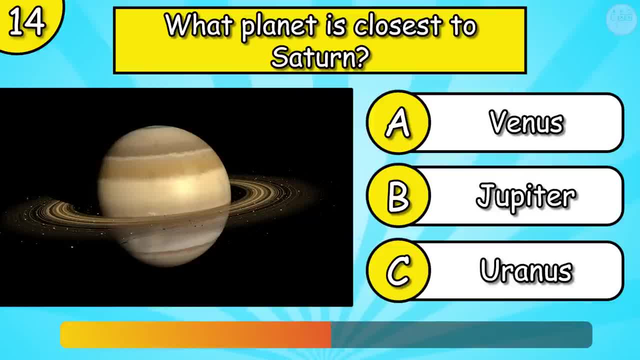 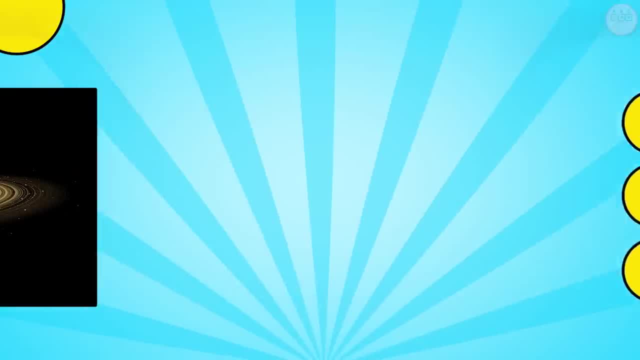 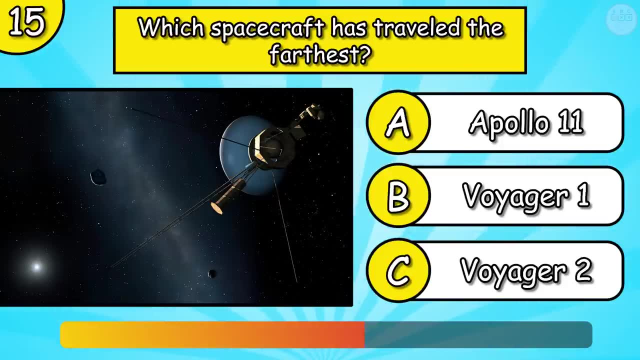 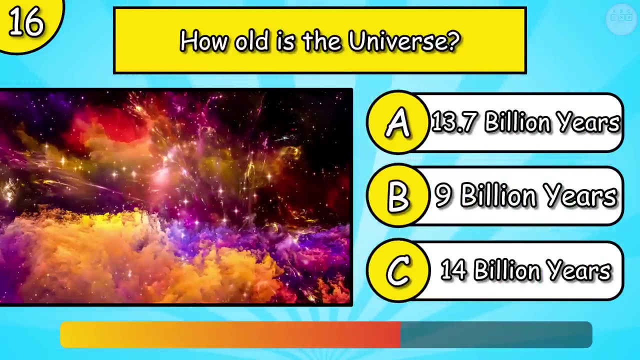 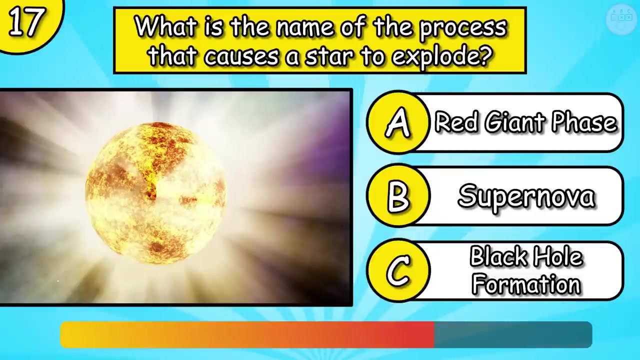 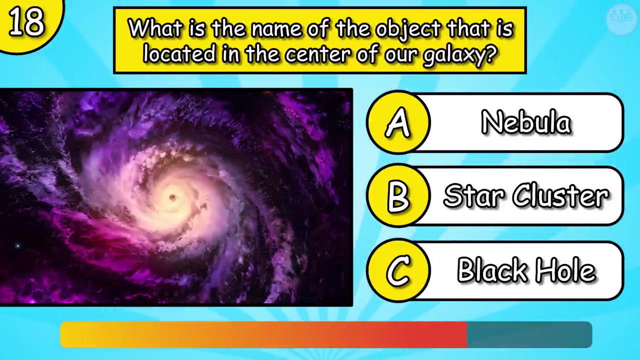 *** Jupiter. Which space craft has traveled the farthest? *** Voyager 1!. How old is the universe? *** 13.7 billion years. What is the name of the process that causes a star to explode? It's supernova. What is the name of the object that is located in the center of our galaxy? 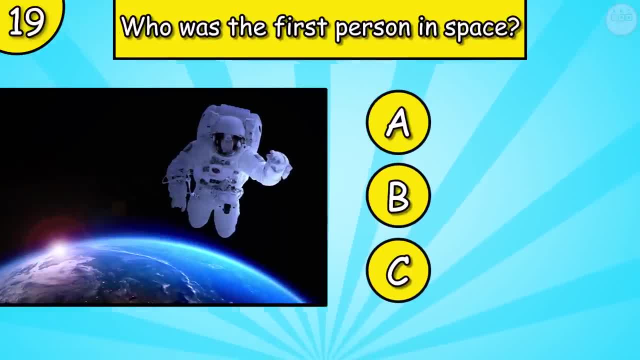 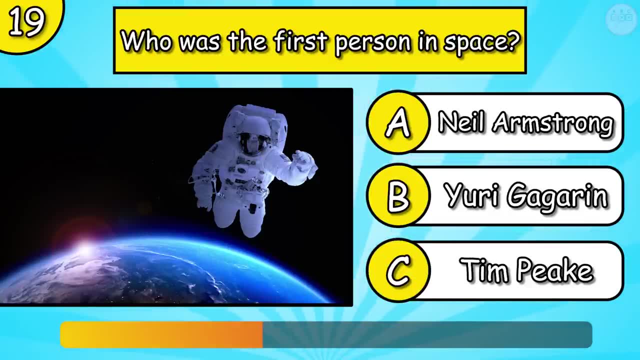 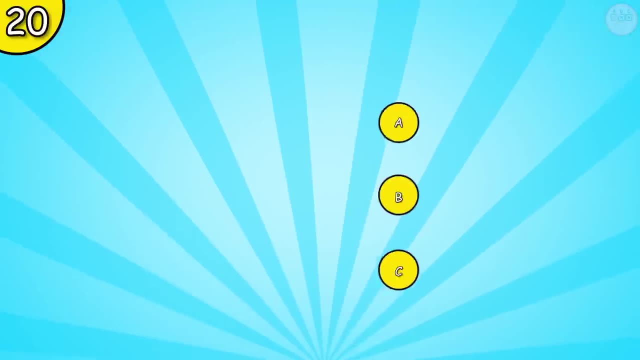 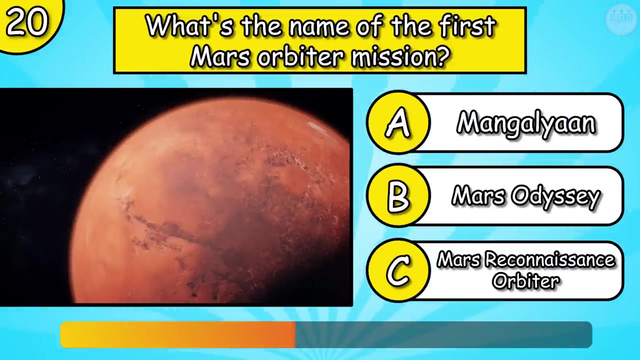 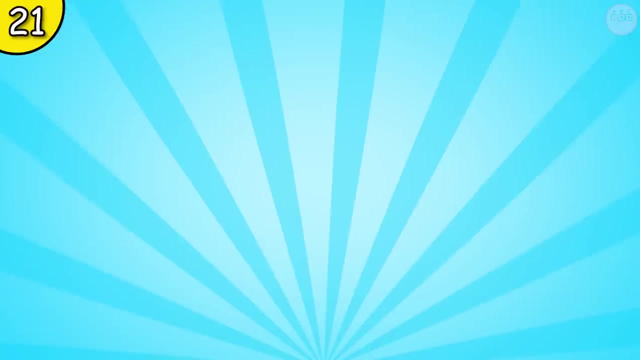 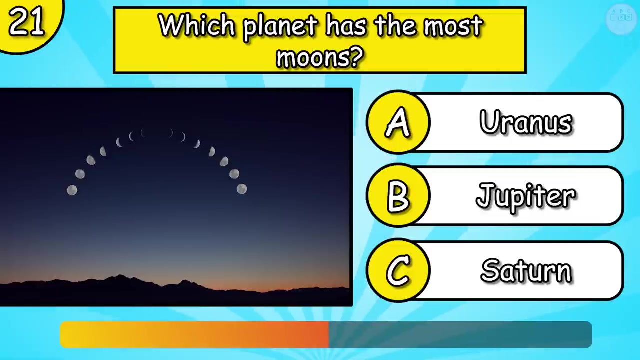 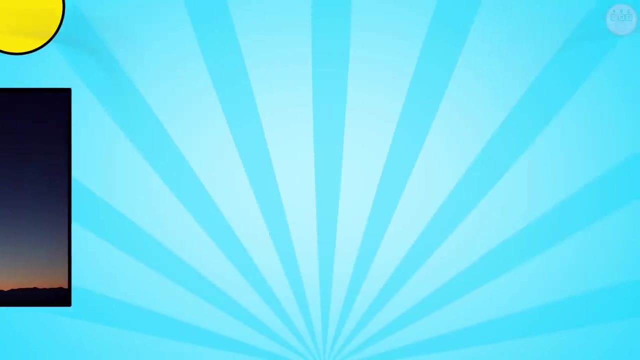 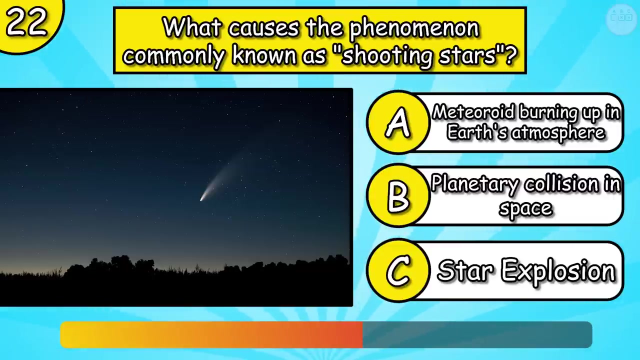 It's black hole. Who was the first person in space? Yuri Gagarin. What's the name of the first Mars orbiter mission, Mangalian? Which planet has the most moons? It's Jupiter. What causes the phenomenon commonly known as shooting stars- Meteoroid burning up in Earth's atmosphere. 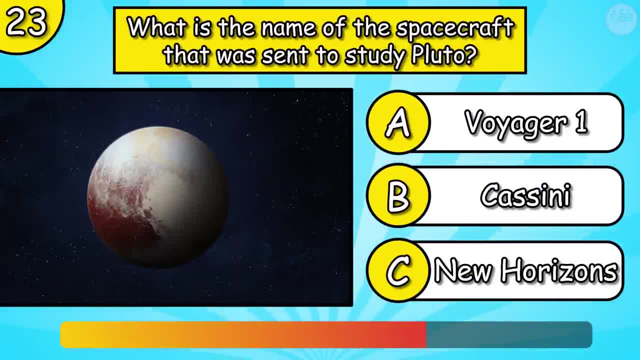 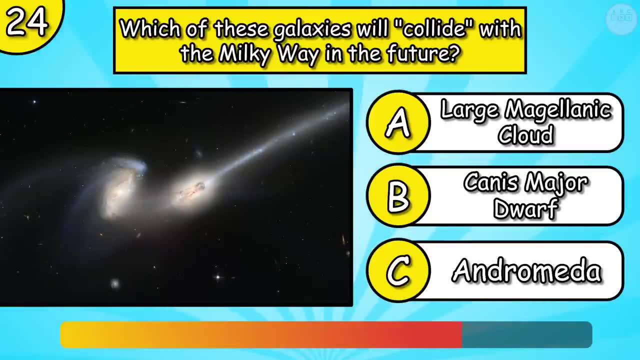 What is the name of the spacecraft that was sent to study Pluto New Horizons? What is the name of the first planet that was sent to study Pluto New Horizons? Some of these galaxies will collide with the Milky Way in the future. It's Andromeda. 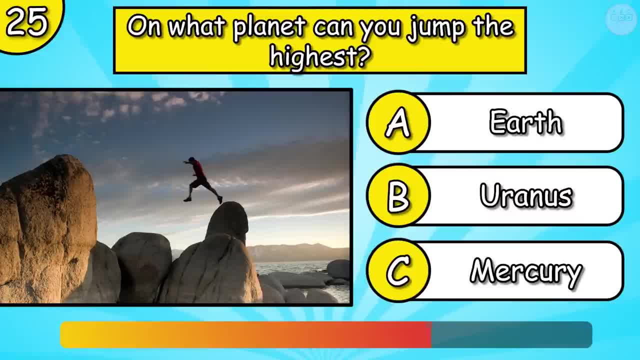 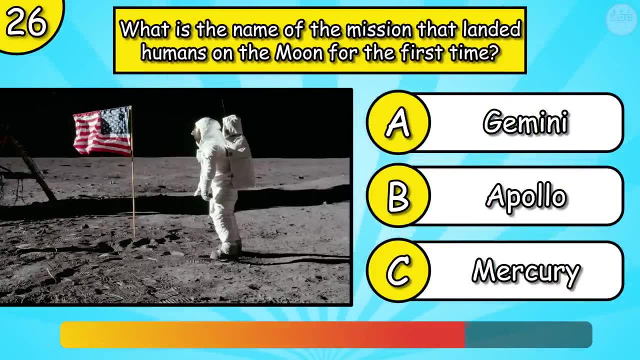 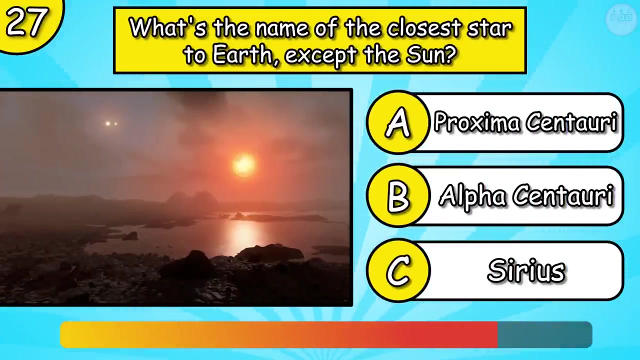 On what planet can you jump the highest? Mercury. What is the name of the mission that causes a star to explode? Mercury. What is the name of the mission that landed humans on the Moon for the first time? Earth? It's Apollo. What's the name of the closest star to Earth except the Sun? Proxima Centauri. It's Proxima Centauri. What is the name of the closest star to Earth except the Sun? Proxima Centauri. Which planet was the first to be successfully visited by a spacecraft? Venus. It was Venus. What is the name of the planet that is often called the Red Planet? 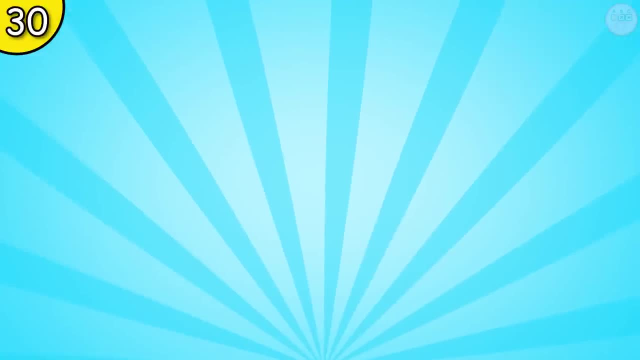 Mars. It's Mars. What is the name of the planet that is often called the Red Planet, Mars? What is the name of the planet that is often called the Red Planet, Venus? What is the name of the planet that is often called the Red Planet? 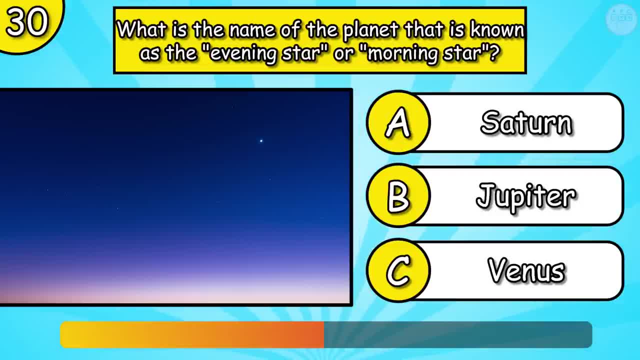 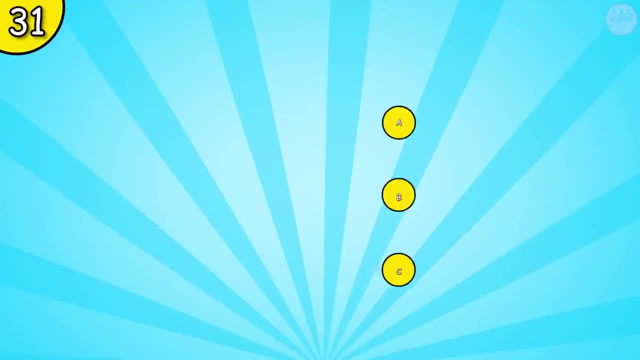 Mars? What is the name of the planet that is often called the Red Planet Moon? What is the name of the planet that is often called the Red Planet Moon? What is the name of the planet that is often called the Red Planet Moon? What is the name of the planet that is often called the Red Planet? 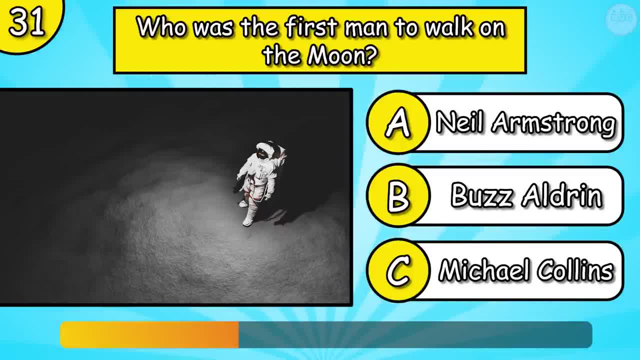 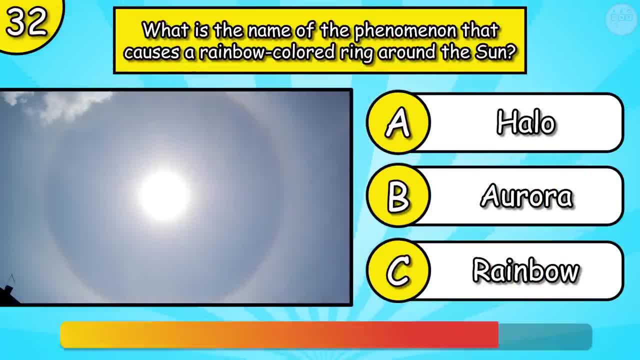 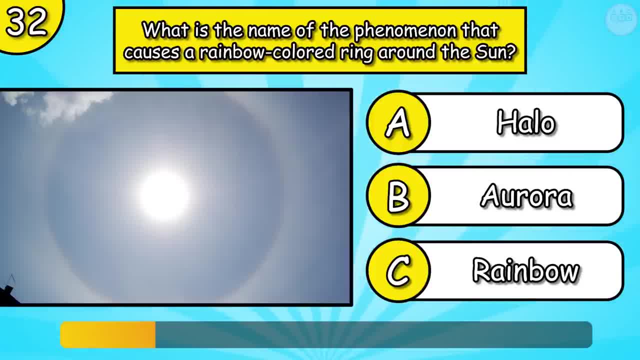 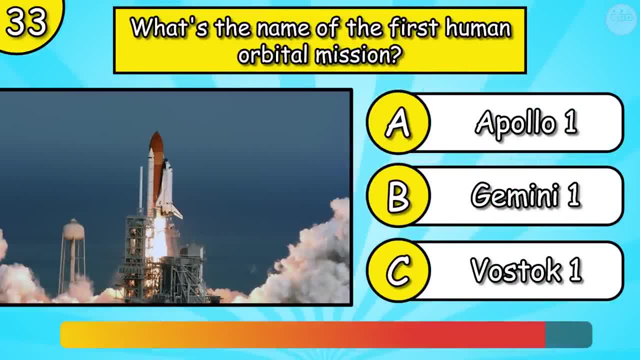